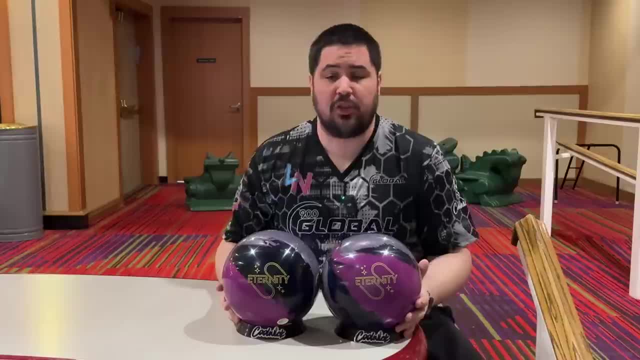 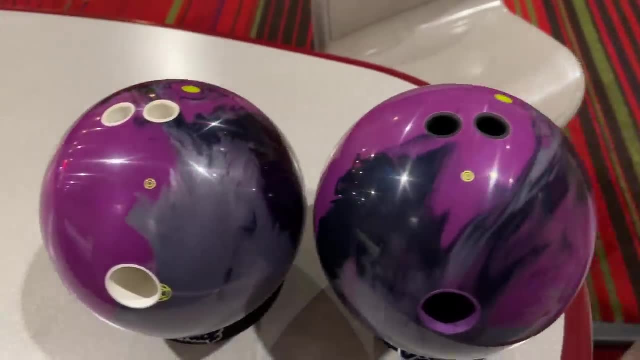 Eternity or anything bowling related. It's a great way to help support the channel, All right, so, as you guys are seeing on screen now, the Eternity that has the black grips is the 15-pounder and the one with the white grips is the 14-pounder, And I went ahead and got the 15-1, undrilled with. 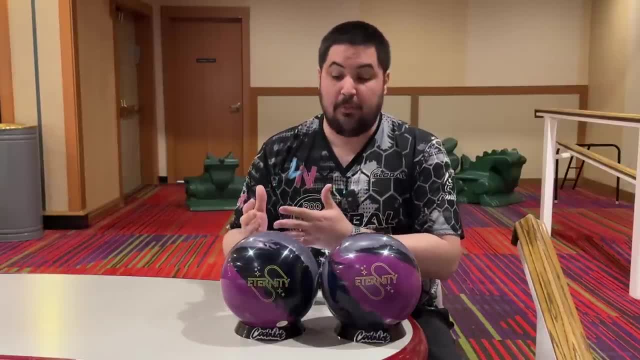 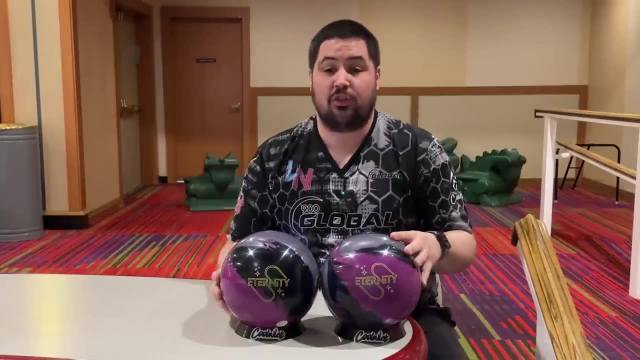 15 pounds two ounces and the 14-pound one is 14 pounds two ounces And I went ahead and got two ounces so that they're going to be a 16-ounce difference, an exact one-pound difference between the two. So there's been a lot of talk recently in the PBA but a lot of pros going from 15 down. 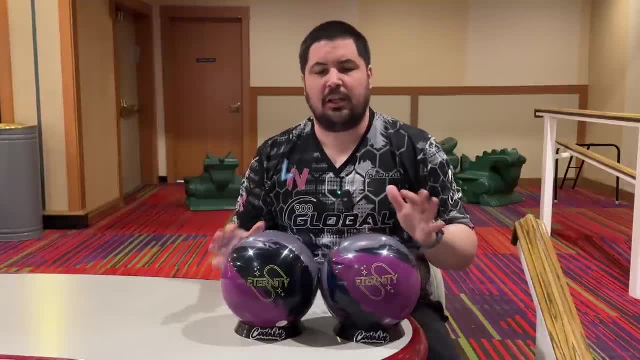 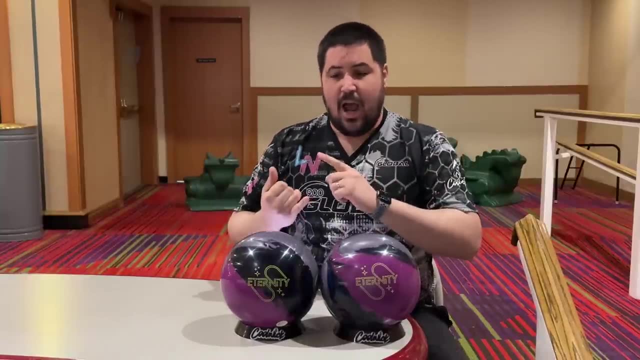 to 14.. And you know we don't have any specto here or anything like that. So we're going to really be taking a look at three things that I want to see if it's at least obvious to the eye. I want to see if the carry percentage is going to be any difference between a 14-pound ball and a 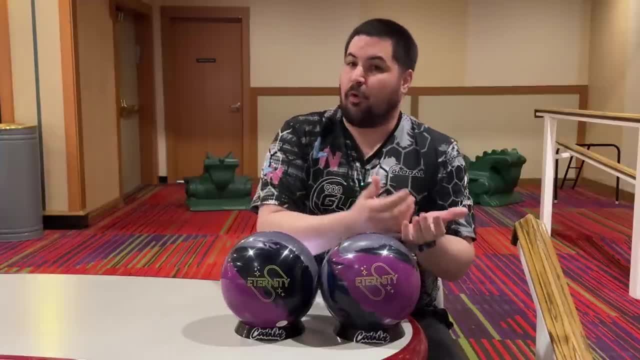 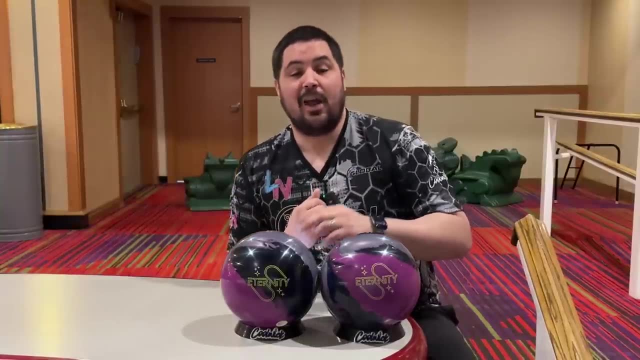 15-pound ball, That one's going to be the tough one, Because if I throw the 14-pound one bad versus the 15-pound one good, or vice versa, that one's going to be a little tough. I am going to write down my speed on every single shot that I throw in 15 and. 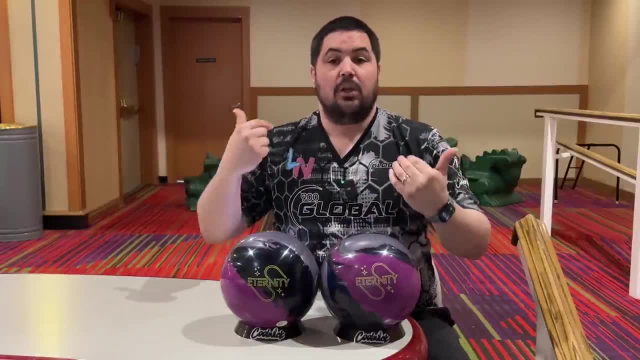 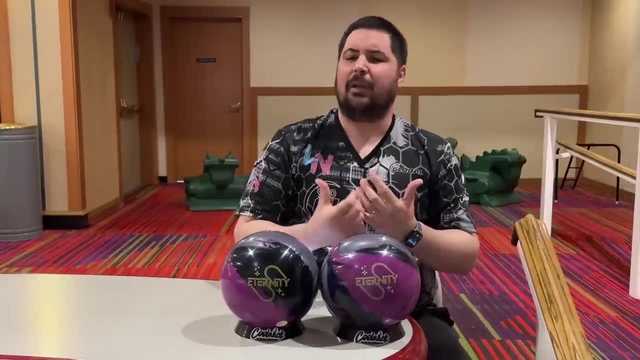 14, so that at the end of the video we can see an average of what the speed difference was, if there is any, between the 15 and the 14.. And then I want to see if the rev rate goes up a little bit with. 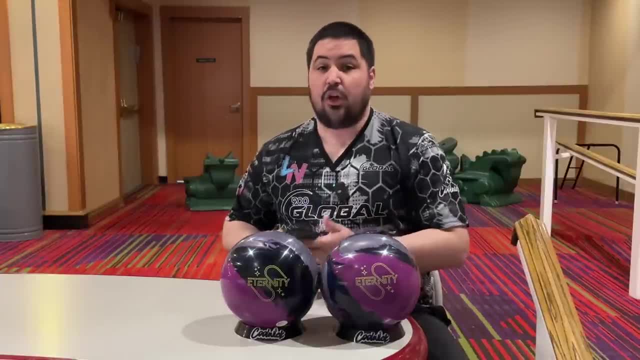 the 14-pound ball versus the 15-pound ball. Now the core numbers are going to be a little bit different, going from 14-pound to 15-pound. So I'm going to go ahead and take a look at that and see if it's going to be any difference between a 14-pound ball versus a 15-pound ball, And that's. 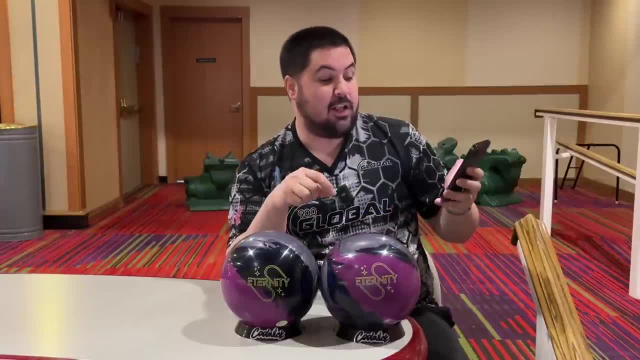 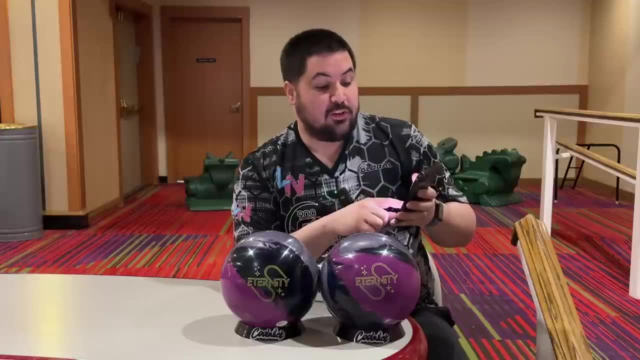 something that we're going to talk about here. The 15-pound Eternity has an RG of 2.49, a max differential of 0.050, and a PSA of 0.014.. Then, when we turn it over to the 14-pound, 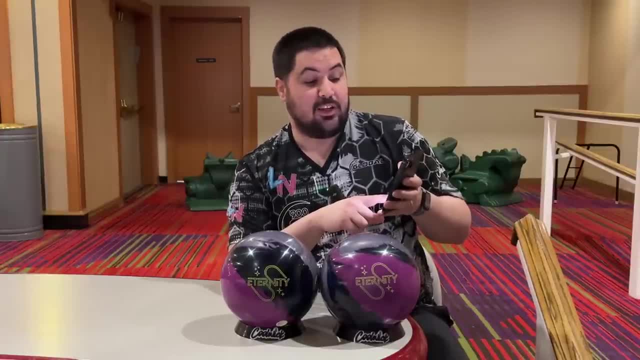 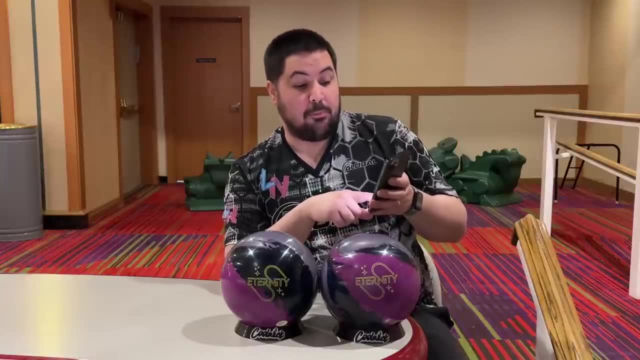 Eternity. it has an RG of 2.51, so it's a difference of 0.02, a max differential of 0.044, so it's going to be lower by 0.006 in the differential and then a PSA of 0.01.. 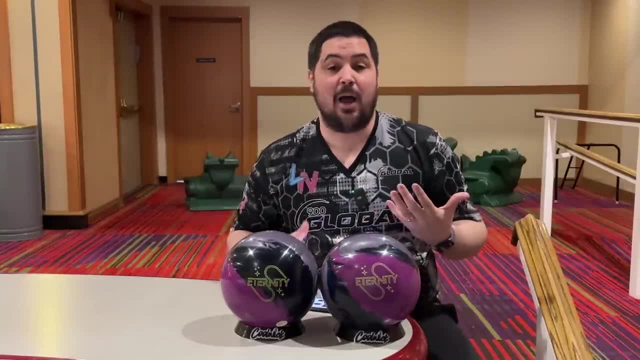 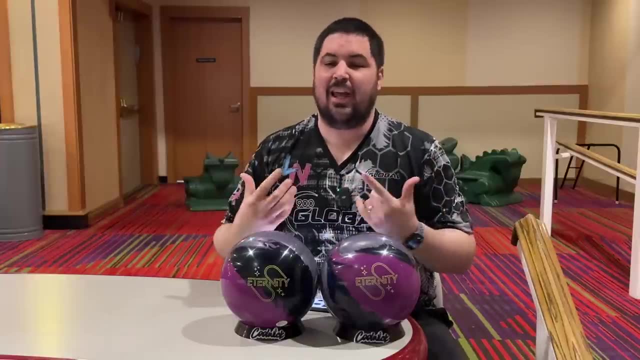 So again, a little different than the 15-pound balls. So the core numbers are going to be a little bit different, but that's really not what we're discussing in this video. What I really want to see, like I said, is there an obvious carry difference between 14 and 15?? Is my speed going? 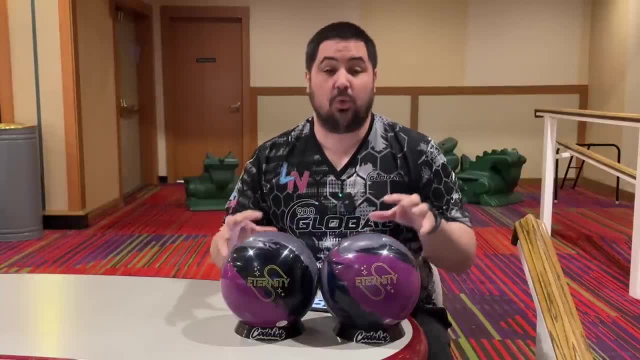 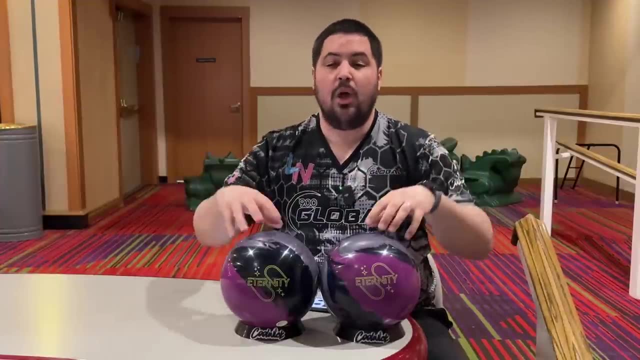 up or down, And is my rev rate going up or down between the two? Let me know down below in the comments if you guys throw 15 or if you throw 14, which one is your favorite, why and what you think the differences are going to be between these two balls. We'll see you in the next video. 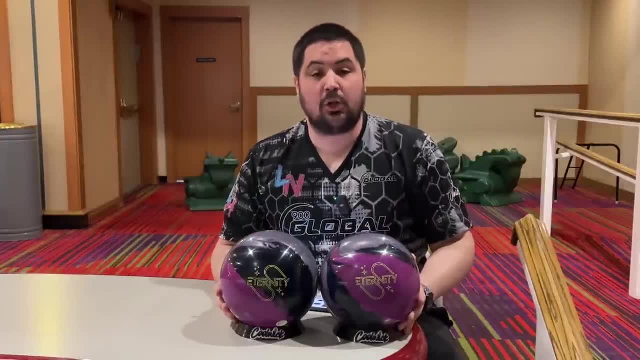 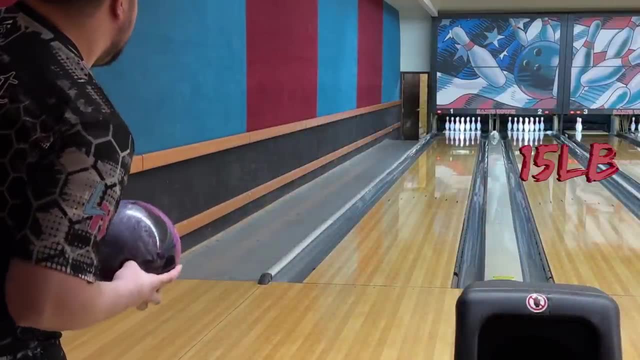 See you guys here on Samstown on lane one on a fresh typical house shot. All right, first shot of the video here. We're going to start in the 15-pound Eternity. We're going to keep track of everything here. 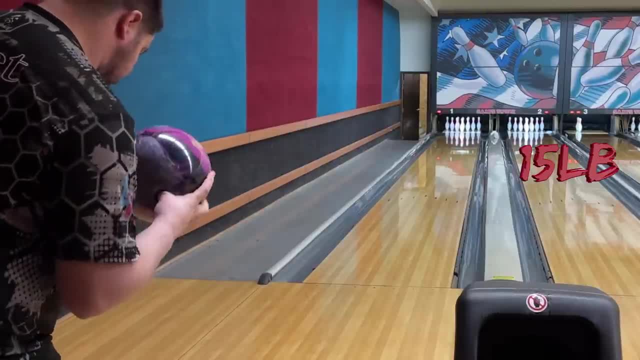 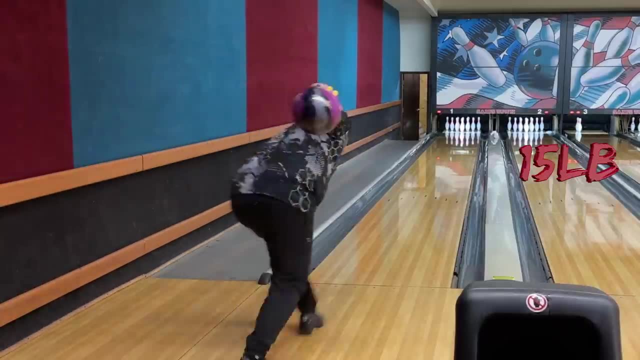 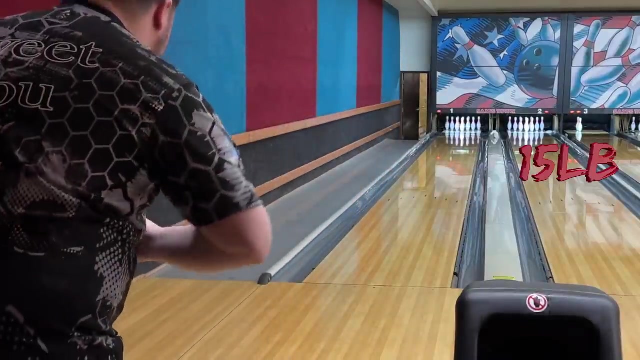 So that last shot I missed in. and when you miss into the oil, that speed is going to creep up. Let's make a good shot here. We'll do one more here with the 15-pounder and then we will make our way into the 14-pounder. 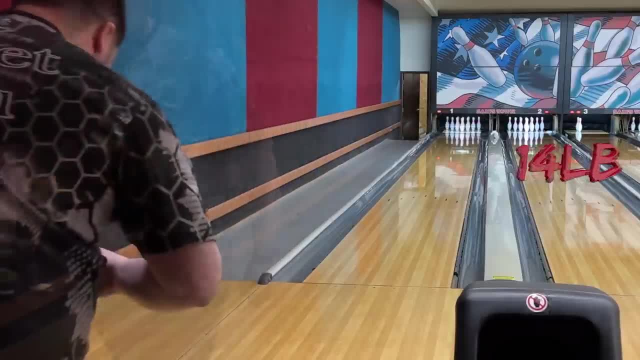 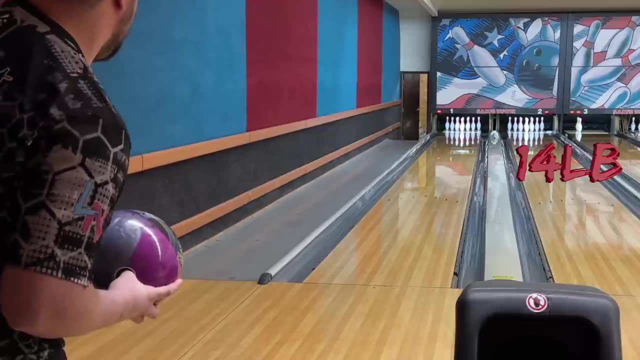 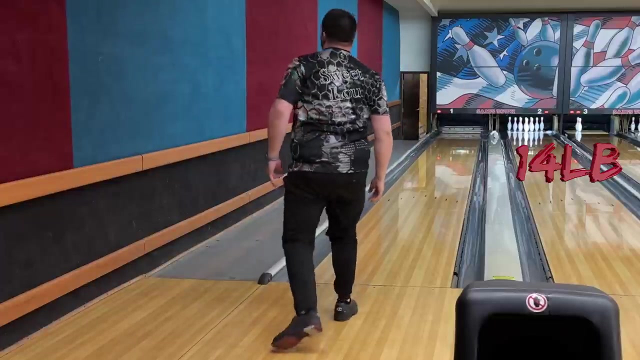 Pretty good shot there, All right. so this is going to be the first shot here on camera with the 14-pound Eternity, and you guys will notice the white grips in this ball. I do feel like with the lower diff on the 14-pound ball. 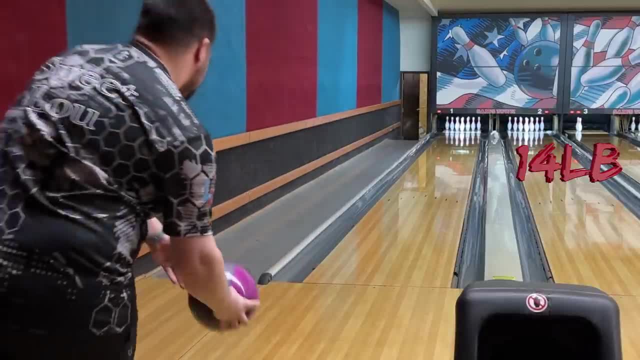 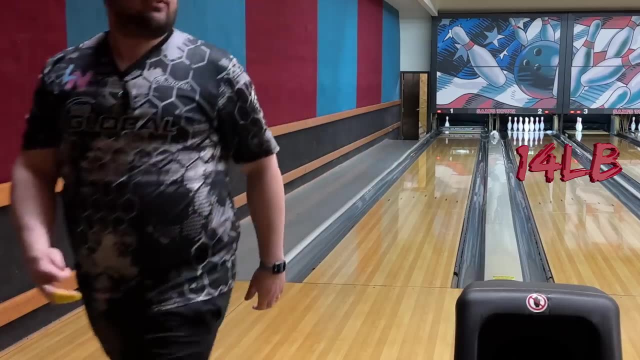 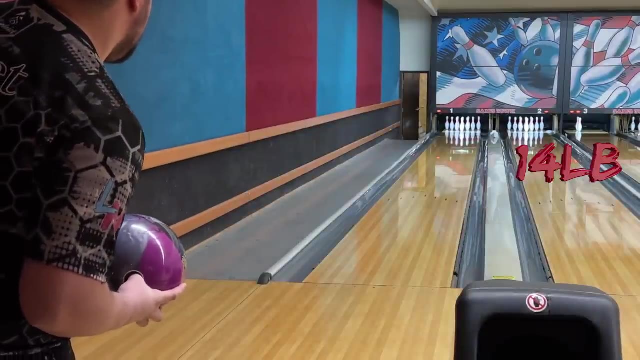 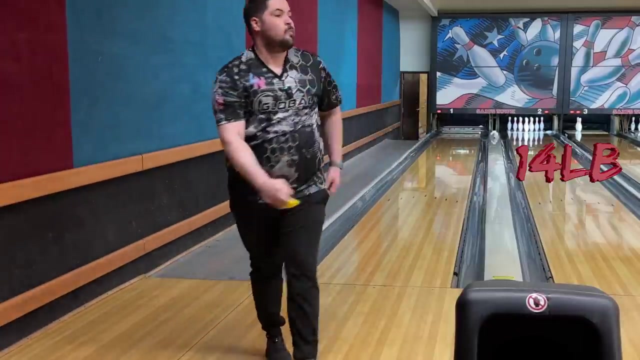 it's making it a little bit quicker down lane. Oh, that's a dirty seven pin. Yeah, seven pin was dirty, but hey, so far no flat tens. Now, obviously this video isn't like super sciencey or anything like that. 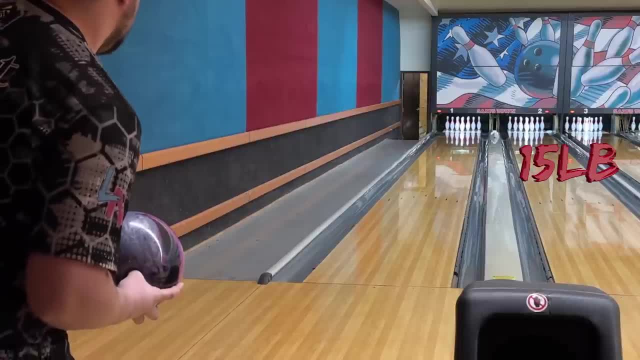 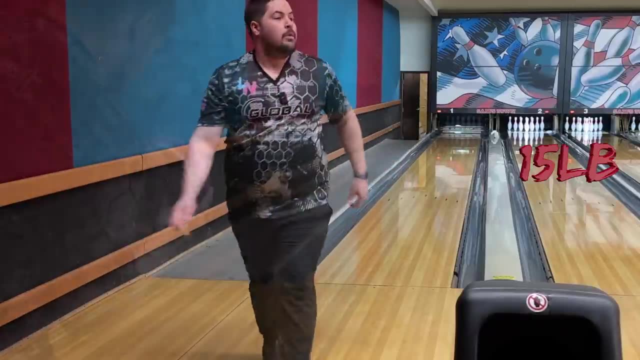 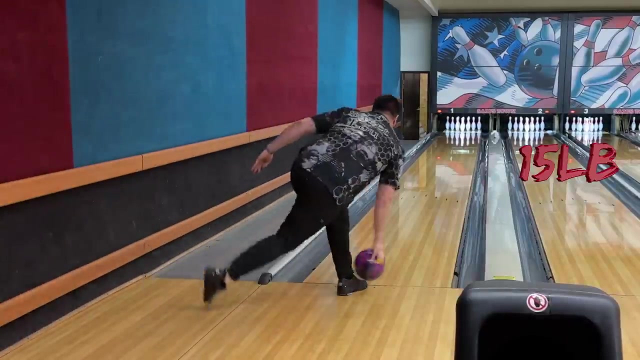 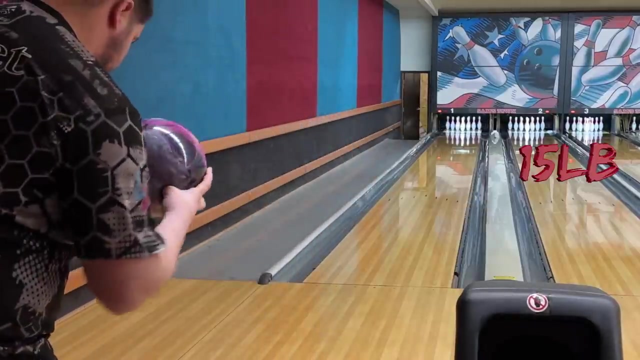 but I think we have some really good stuff here to share with you guys. Again, let's just keep making quality shots here. Missed that one, right? Wow, that clip shouldn't even be added into everything here, but we show every shot, no matter what. 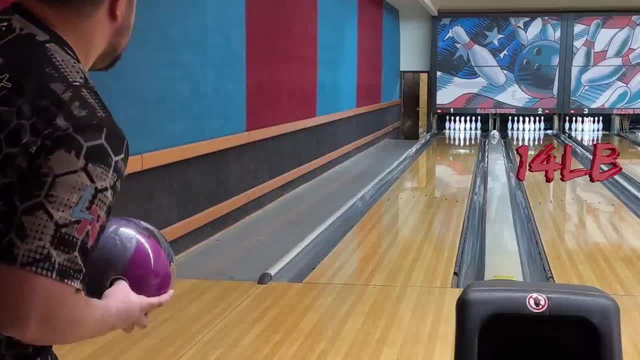 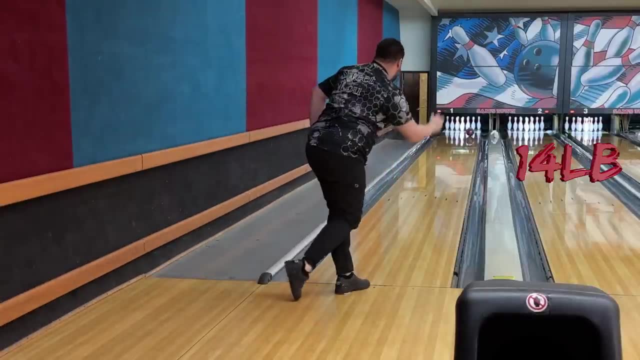 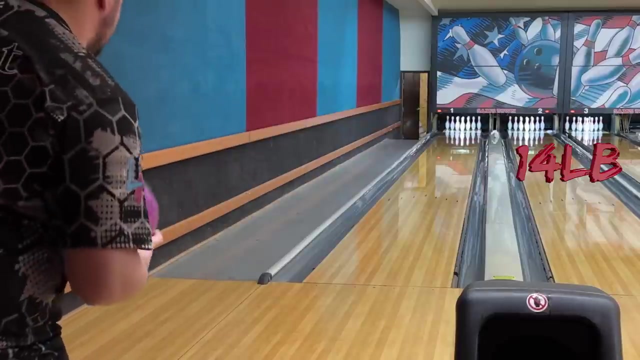 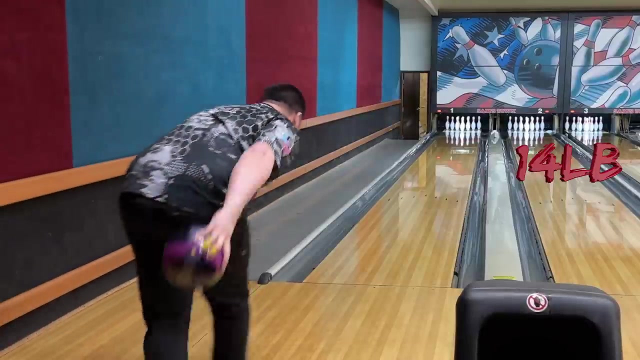 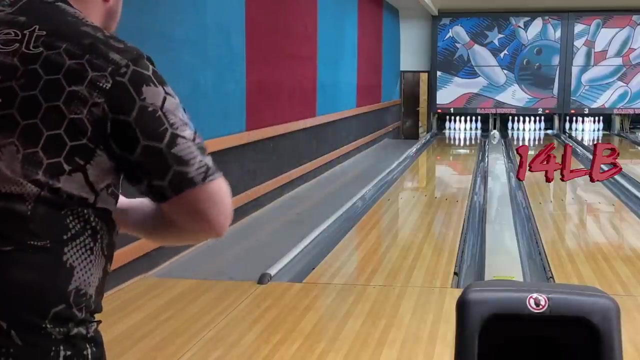 All right back into the 14-pound ball. That's amazing. That last shot was interesting. It was actually one of my slower shots of the day on a really good shot with the 14-pound ball. So those last two shots are really interesting because they don't feel like I'm throwing them. 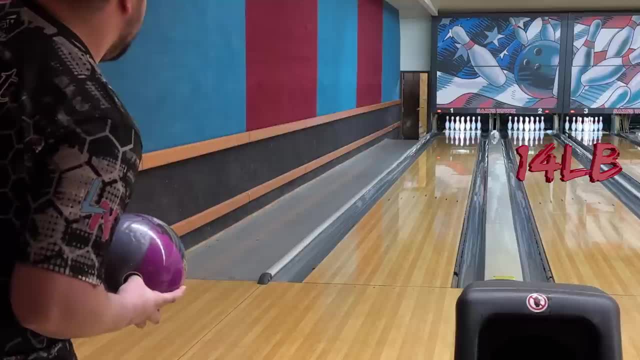 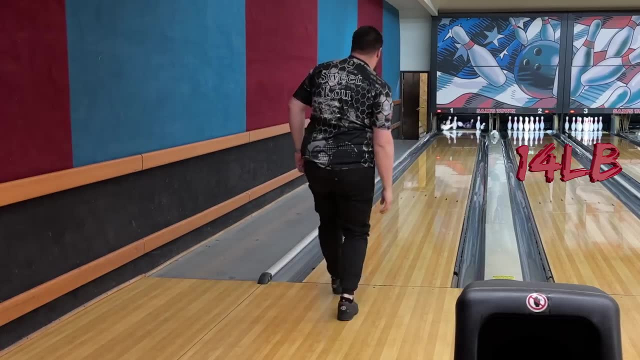 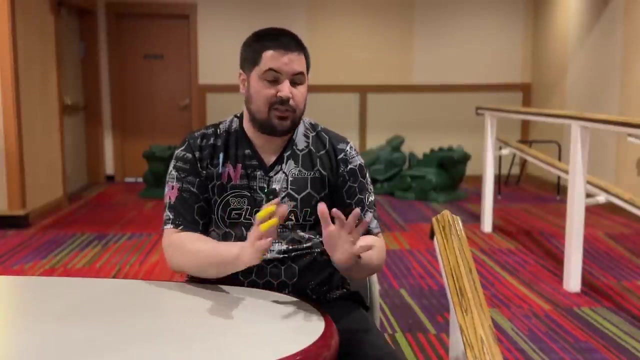 slower. They feel like really, really good shots and they've been sub-15.. All right, so this is some pretty interesting stuff that we've gathered. It's only been 12 shots, six with each, So I'm going to really wait till the end of the video to show you guys the full 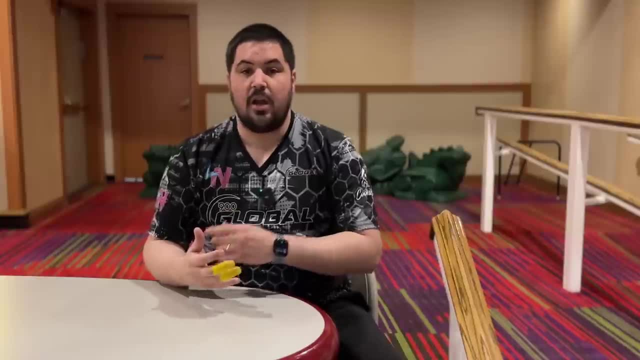 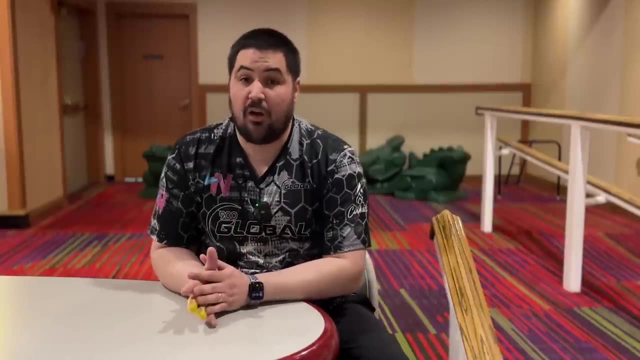 speed differences. I'm keeping notes here, shot to shot, keeping track of my speed, keeping track if it was a good shot or a bad shot, what the result was And so far. it is pretty interesting And I want you guys to pause the video here for a second. 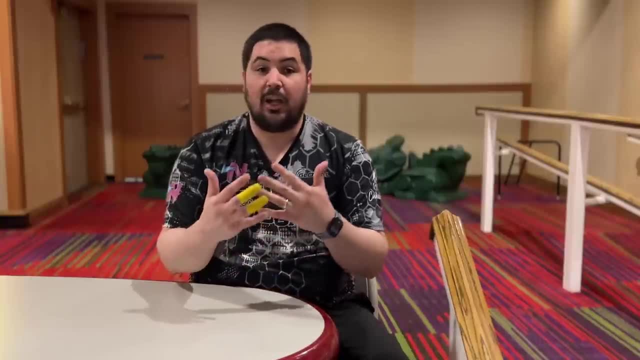 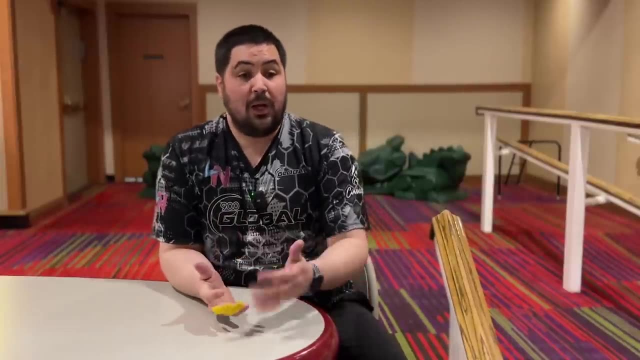 and write a comment down below and let me know if you were expecting the results that you're seeing so far, or were you thinking that they were going to be completely different? So we're going to get back on the lanes And, like I said, this is not a ball review. We're 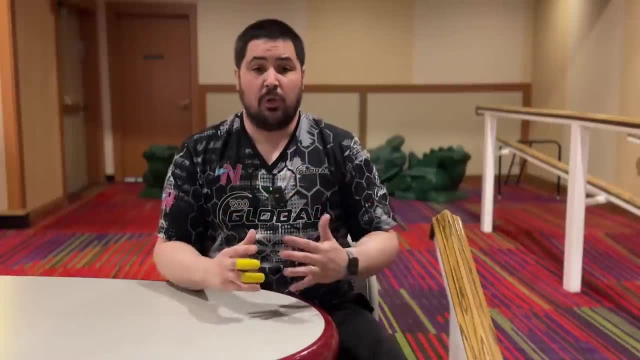 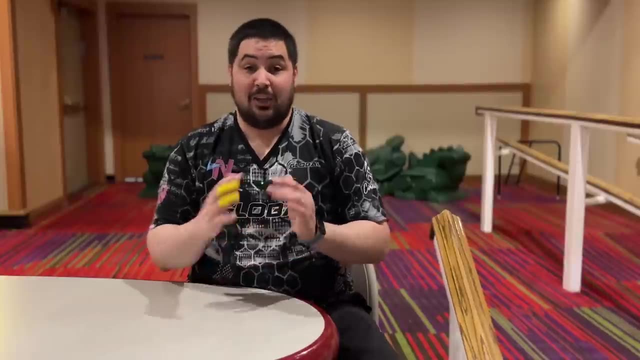 not reviewing the Eternity. We already know that the Eternity is a really good ball. This is more so just seeing what the differences are between that 14-pound and the 15-pound ball. And so far I think that my execution has been really good, except for that one shot that I leaked right. 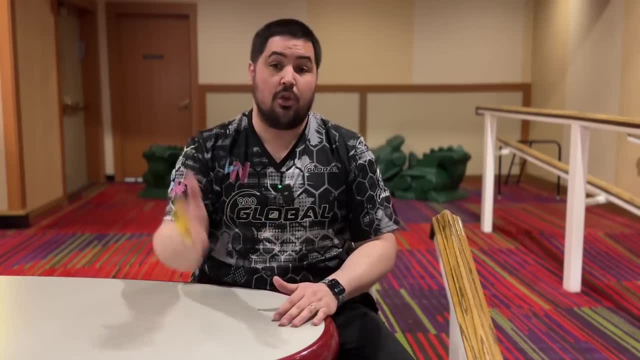 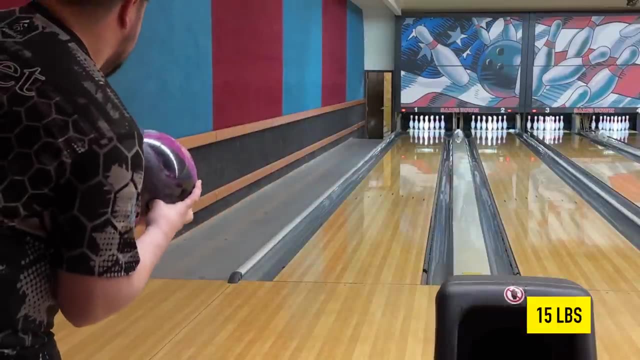 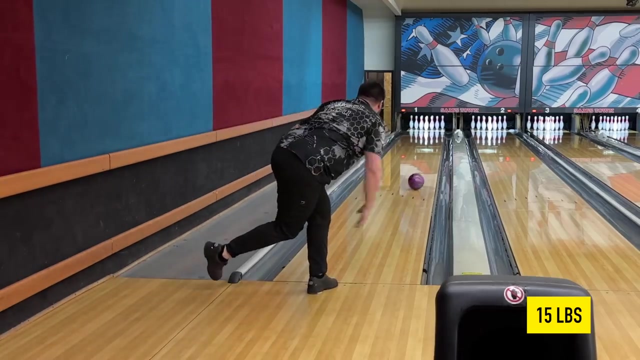 And so that one's going to maybe throw off the numbers a little bit, but we're going to show you every single shot, as always. So let's get back on the lanes here, All right? second group of shots here, back into the 15-pound. Eternity Missed right again on that one. I mean so far I've. 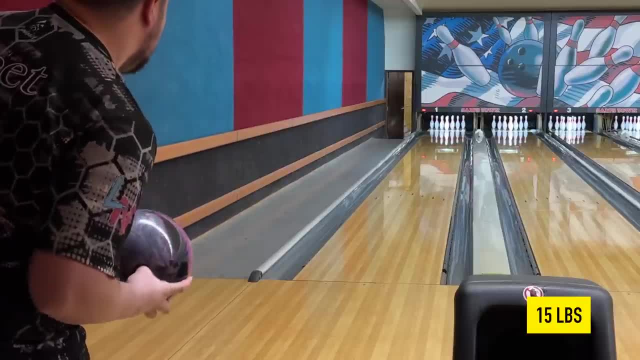 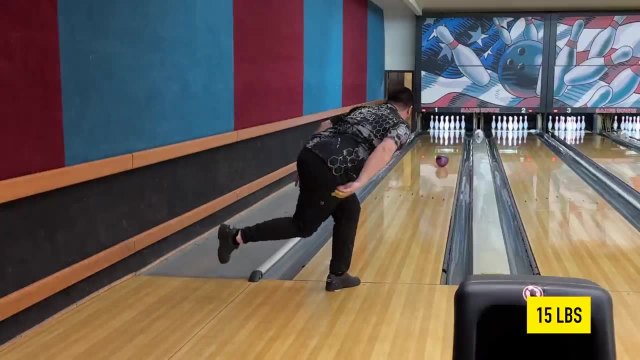 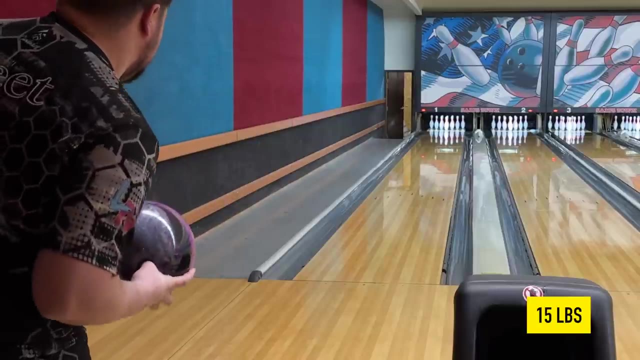 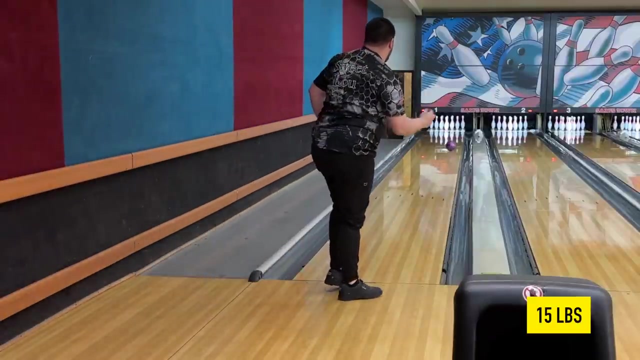 thrown more bad shots with 15 than I have with 14.. Let's see if that finishes that way. One more shot here with 15, and we'll get back into the 14-pounder. Oh, threw that pretty bad. All right, now back into that 14-pound Eternity. 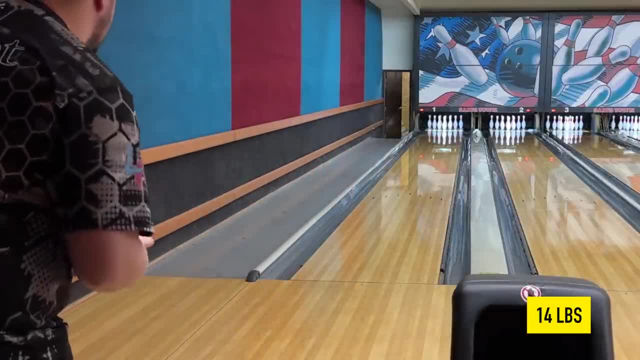 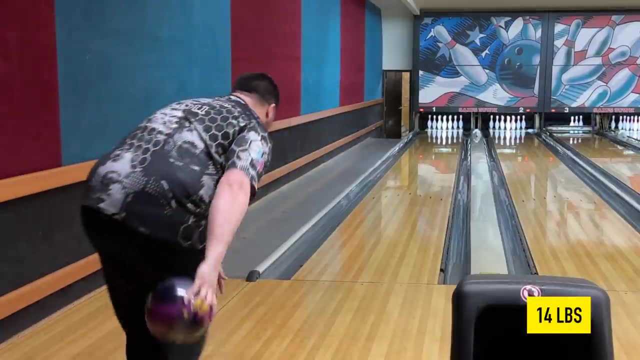 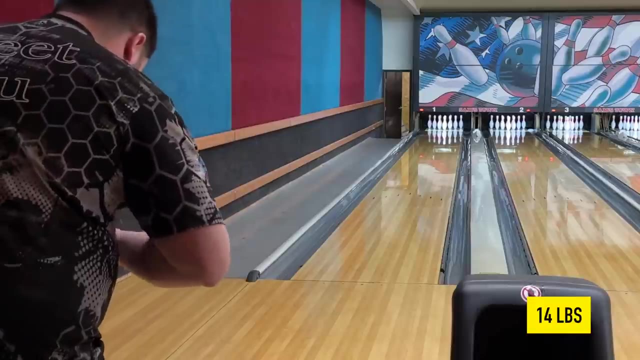 I do think that this 14-pound one hooks a little more down lane a little longer, a little bit more pop down lane. That last shot there I moved one left of my feet. I forgot to tell you guys. so this is going to be still that one board move left. 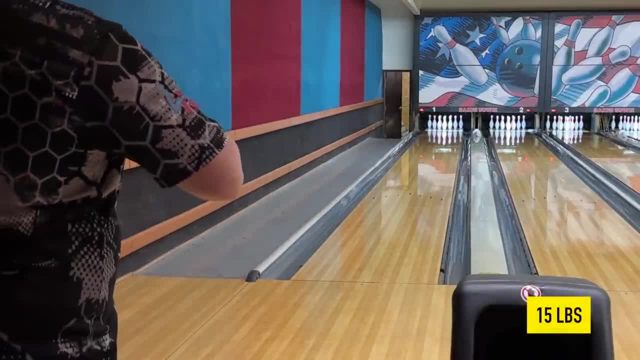 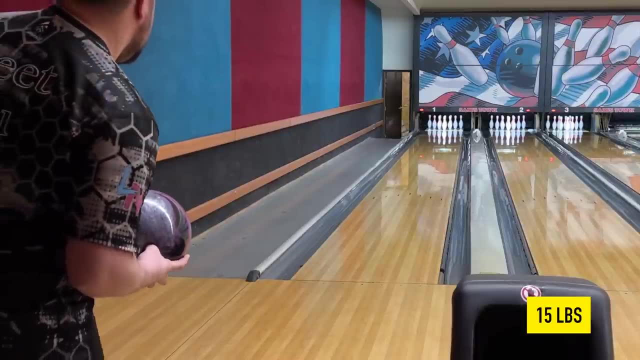 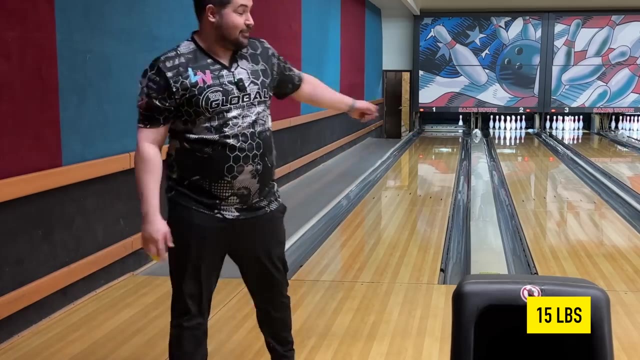 Oh, all right, back in the 15-pounder. We're going to go to that same spot that we just blower 9-pinned with the 14-pound ball. Oh see, that's interesting. All right, so I'm going to move back right with the 15-pounder. 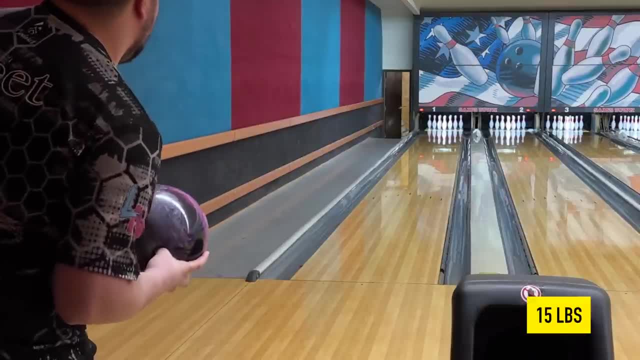 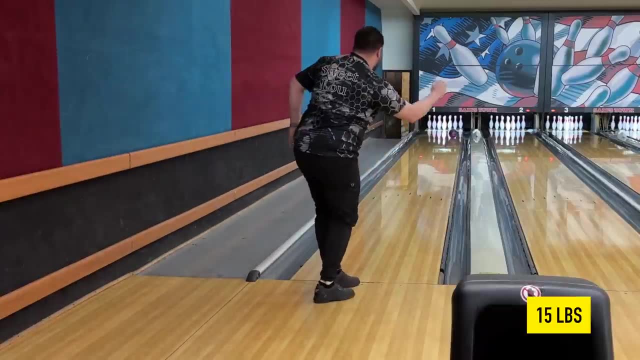 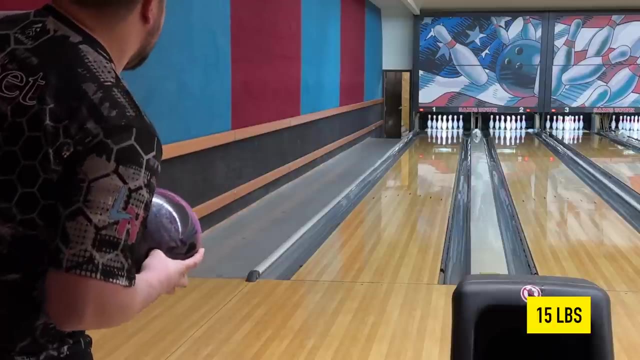 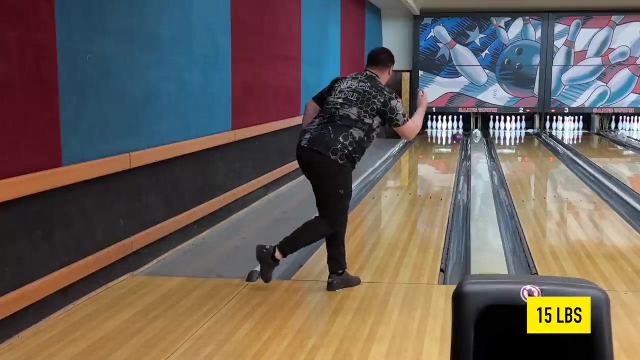 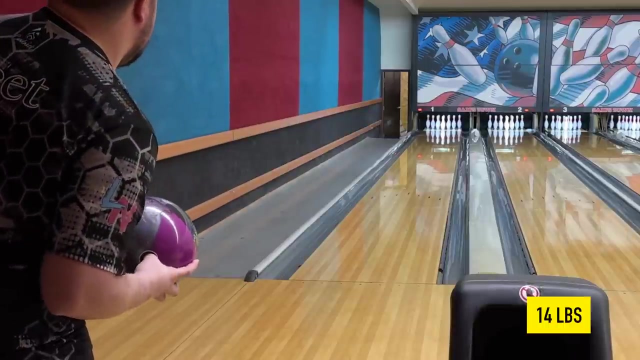 That was a very interesting little flat 10 there. All right, so I am noticing that the 15-pound Eternity is allowing me to stay straighter longer. All right back into the 14-pound Eternity. Let's just continue to make good shots here. 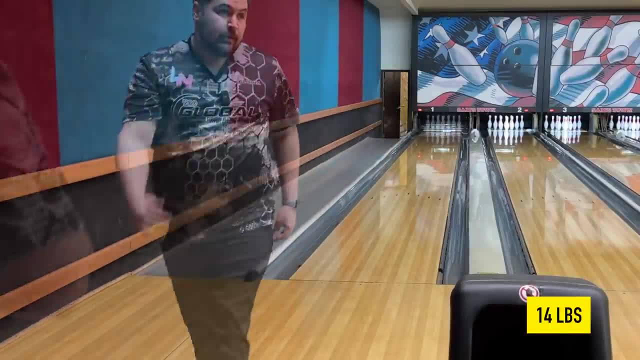 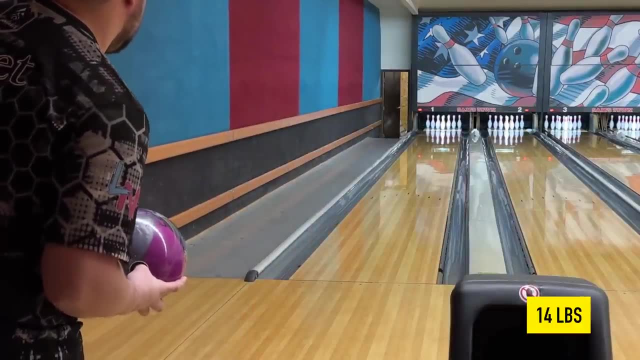 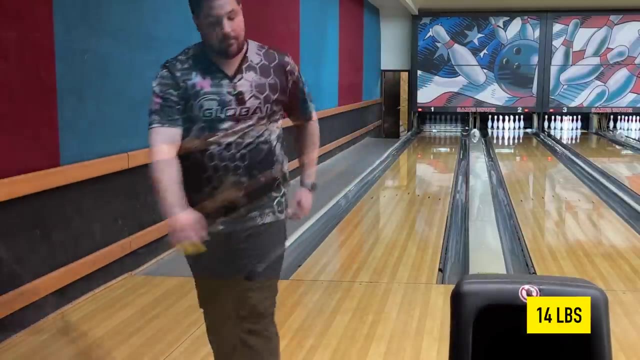 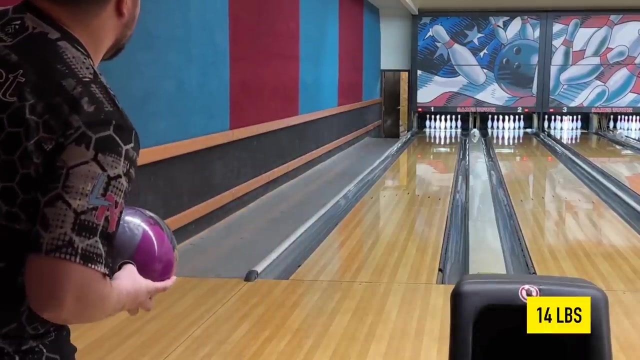 You guys will see the results here at the end, but I'm pretty impressed- Honestly kind of shook- by the results I'm seeing so far. The lanes are definitely starting to tell me to move, so on the next group of shots we'll chase both of these balls in a little bit. 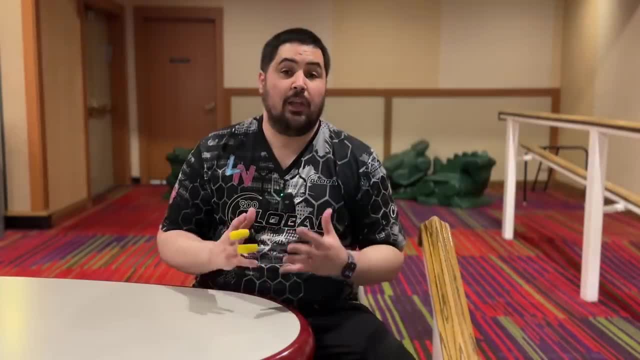 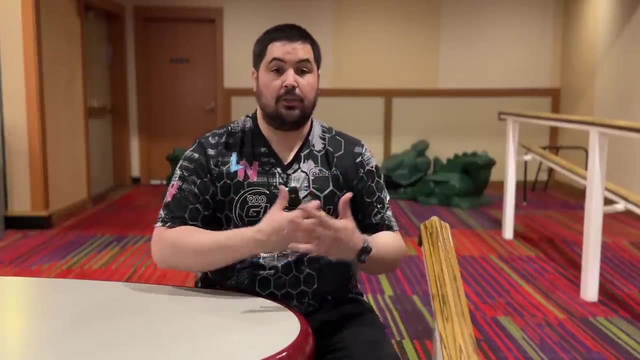 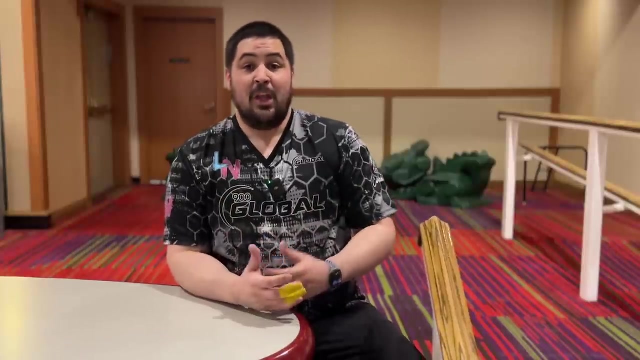 See it Go All right. so last break here, and I kind of want to stop for a second and talk about ball motion. when comparing this 14-pound ball to the 15-pound ball, specifically about the Eternity, because it's the only 14-15-pound ball combo that I have, The 14-pound Eternity for sure feels like. 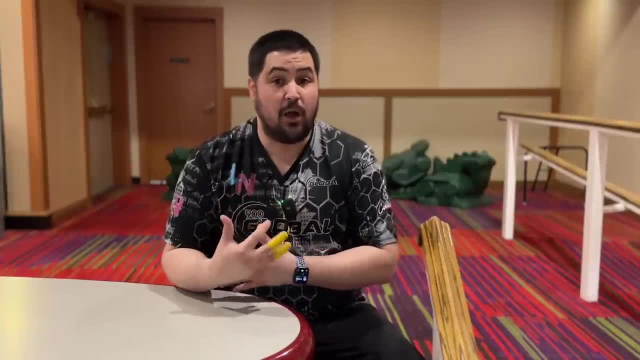 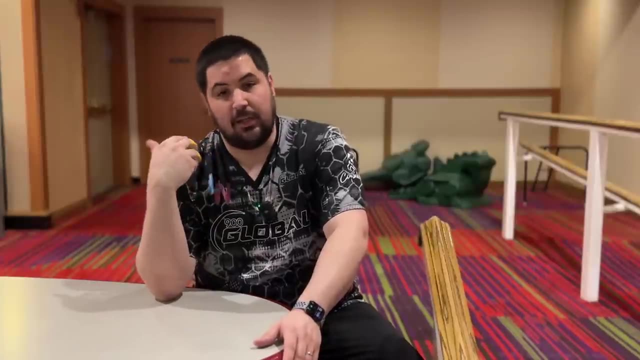 it's a little bit cleaner through the fronts, a little bit more responsive down lane when compared to that 15-pound Eternity. Now, it's not always going to be the case. There are some balls and you guys are just going to have to do your own research on this, but there are some balls. 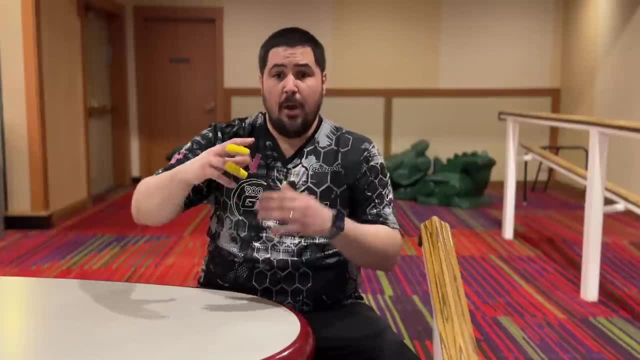 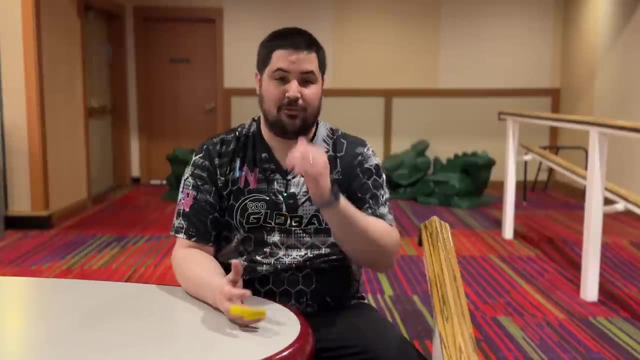 where the differences between 14 and 15 are bigger than this Eternity. but there are also some that are more similar, like the numbers don't change much from 14 to 15.. Balls like that Exotic Gem- I think it's another one that I was looking at to. maybe I was deciding between the Exotic Gem. 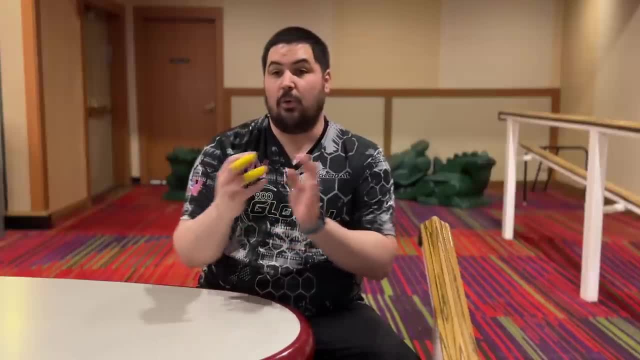 or the Eternity and the Exotic Gem. I think the numbers in 14 and 15 were much closer than the Eternity. so just keep that in mind, that going from ball to Eternity it's going to be a little bit different. I think it's going to be a little bit. 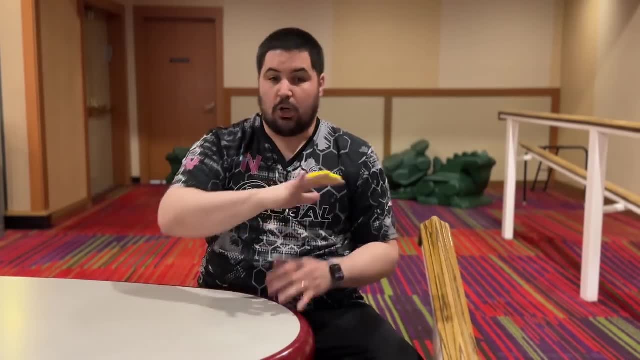 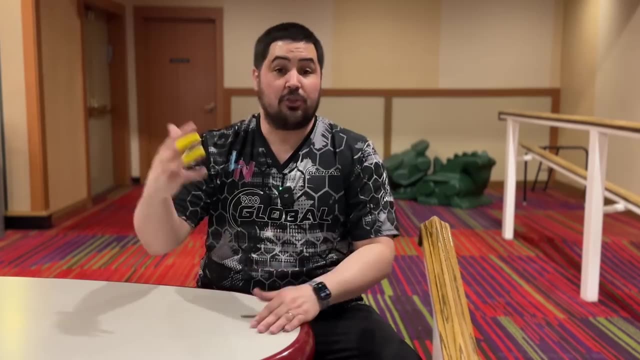 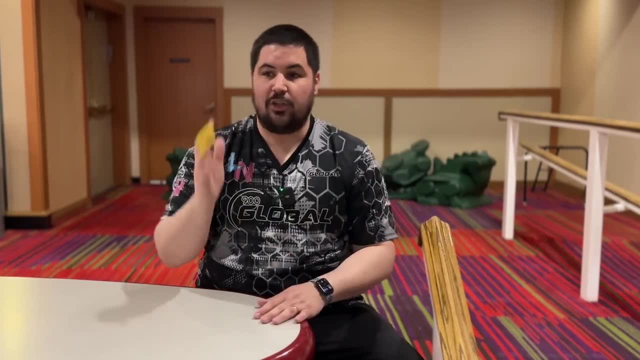 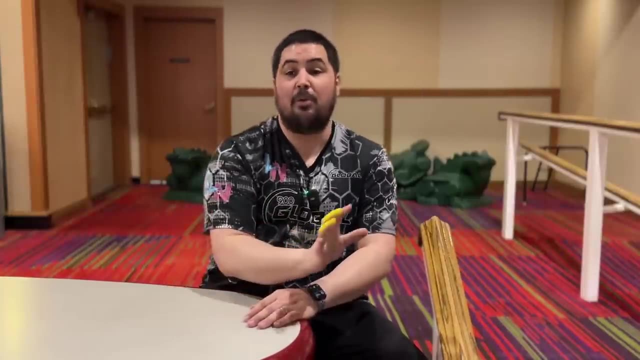 you go from ball to ball to ball. So the core shape doesn't matter, just the numbers are what actually matter. So let's get back on the lanes and I'm going to chase both of these, the 14 and the 15-pound. I'm going to chase them both left a little bit, especially that 14-pound one. 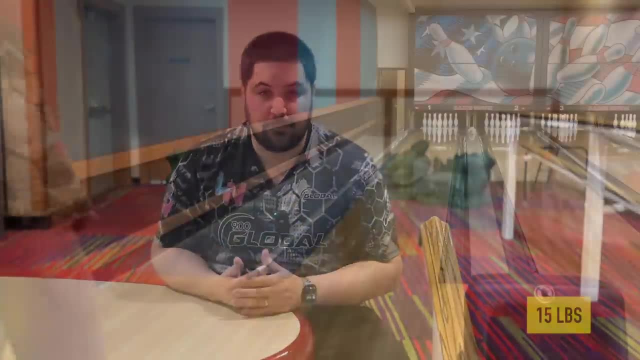 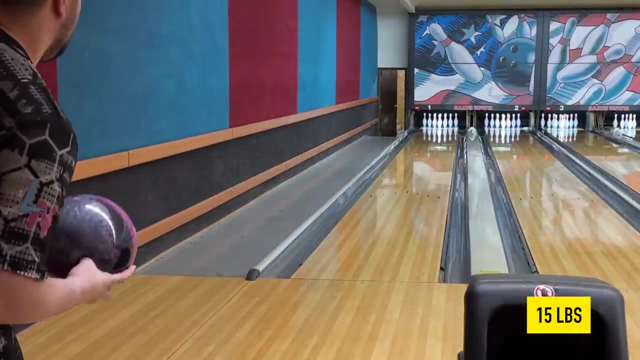 because I think it's telling me to start creeping in and creating that shape. All right, this is 15 pound eternity. we're just going to take an arbitrary move left here, so it'll be about 10 left of both of them, just to see how they look from a little bit further in. 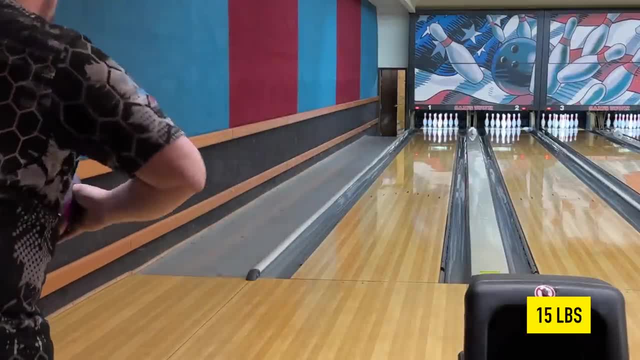 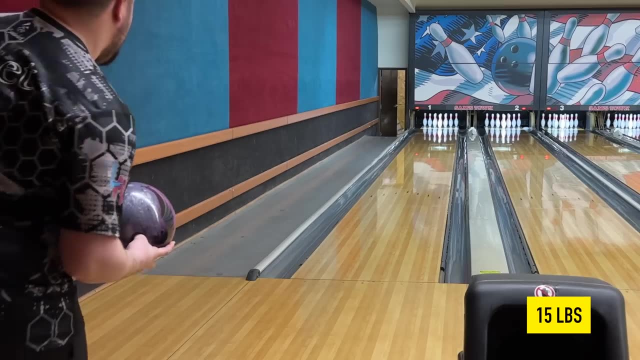 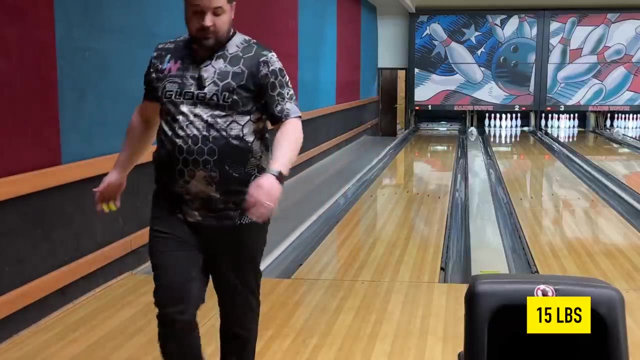 That looked pretty good. So these shots from here with both of these balls are going to be a little slower, because we're doing our little slow hook trick that we like to do. Nice kick of the 10.. All right, now one more here with the 15 pound eternity. 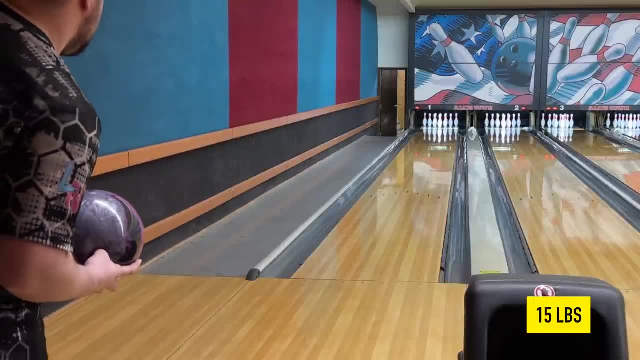 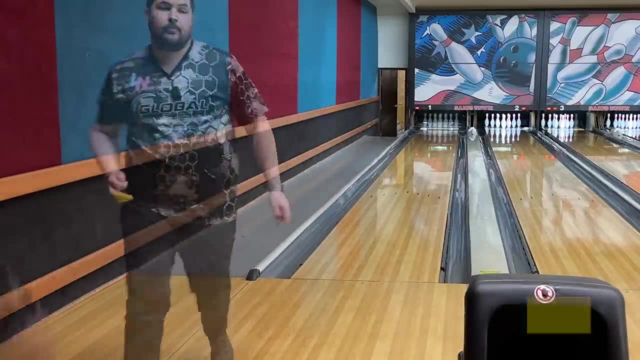 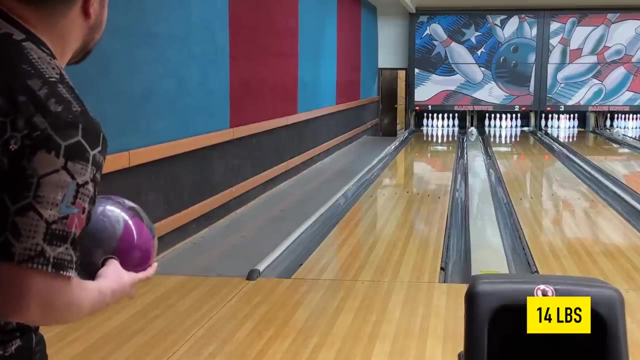 This is my favorite trick, by the way: just slow hooking it. Yeah, this is going to be really interesting because I feel like it's easy to slow hook the heavier ball, but we're going to see This is the same spot with the 14 pound eternity. 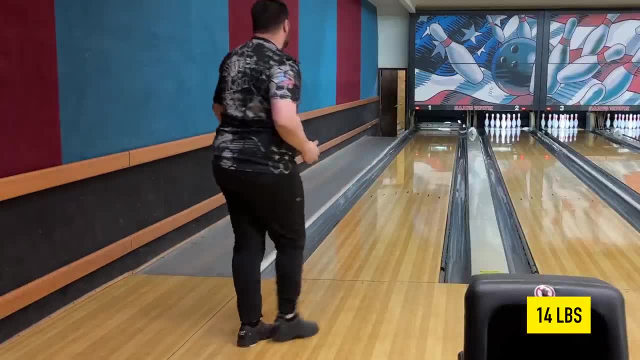 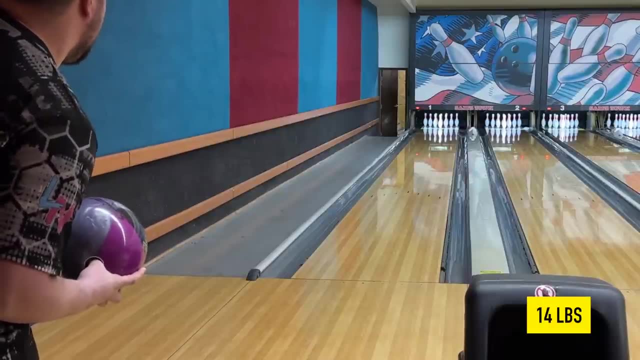 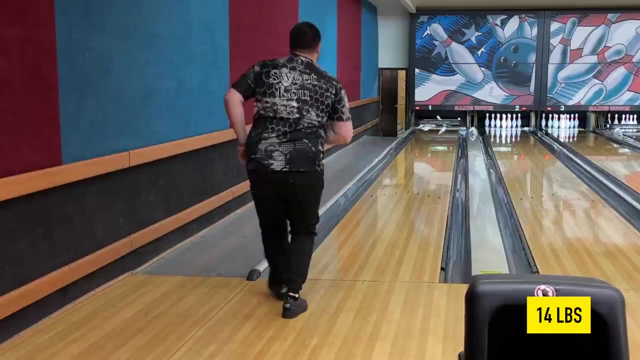 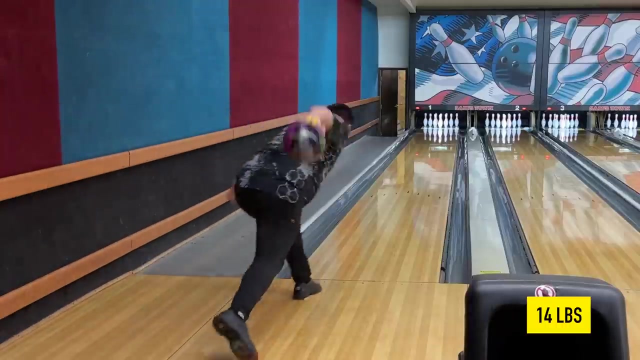 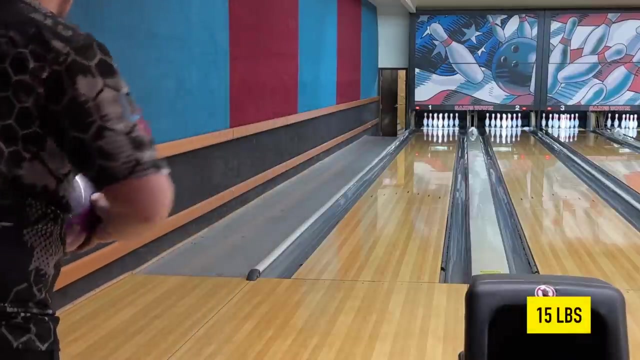 Yeah, I definitely feel like it's harder to slow hook this lighter weight ball. I mean, just after one shot, Let's try again One more from here with the 14 pounder. See it All right back to the same spot with the 15 pound ball. 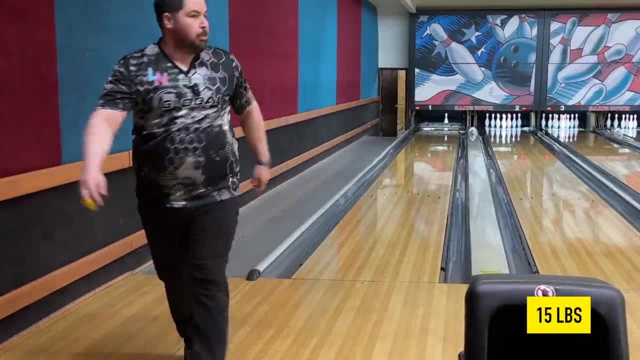 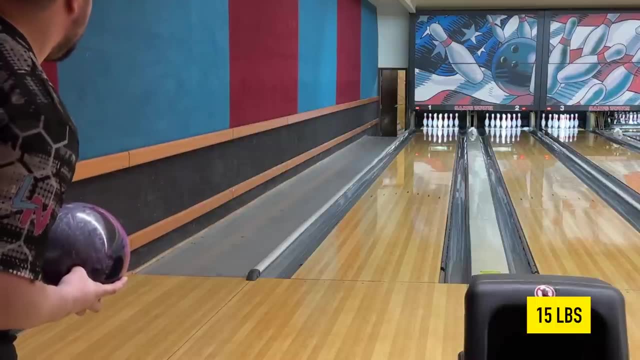 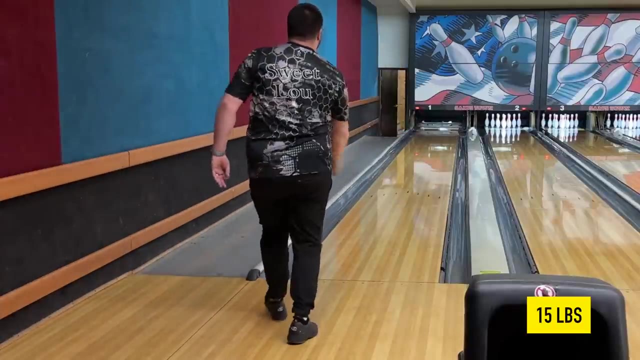 Oh, I missed in a little bit there. Blower nine. All right, definitely don't want to miss in like that. Let's make sure we get it going to the friction a little bit. Oh, and then I shove it right, Wow. 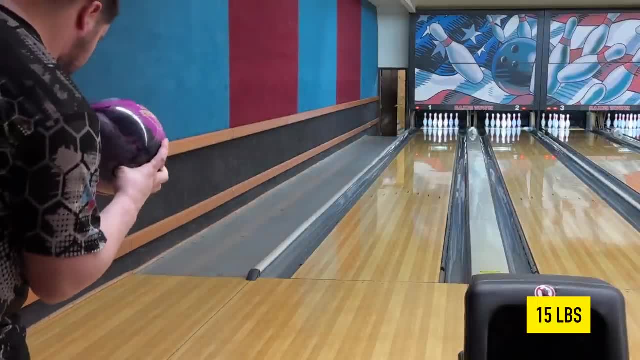 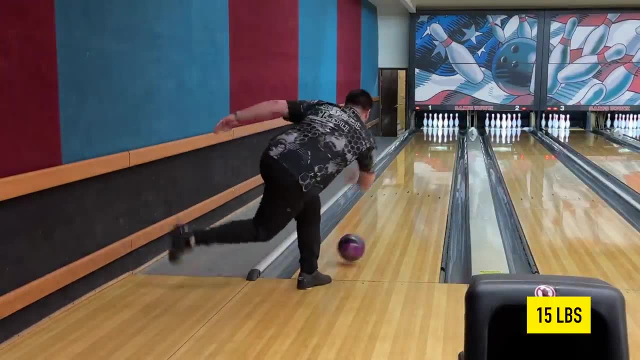 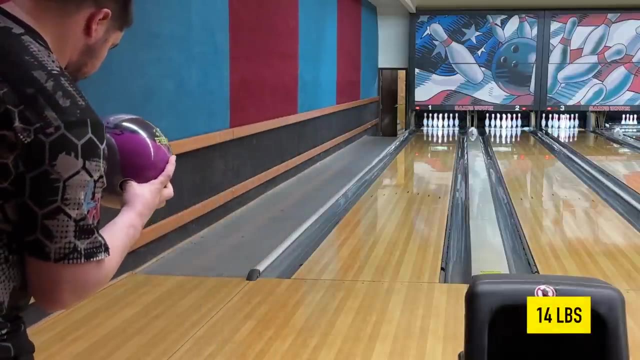 All right, last shot, Last shot of the video with the 15 pound ball. Let's get in between those two shots there. There we go. All right, last shot of the video, or the last three shots of the video, all going to be in the 14 pound eternity. 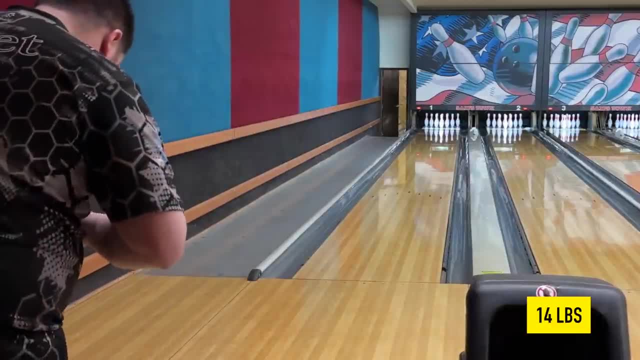 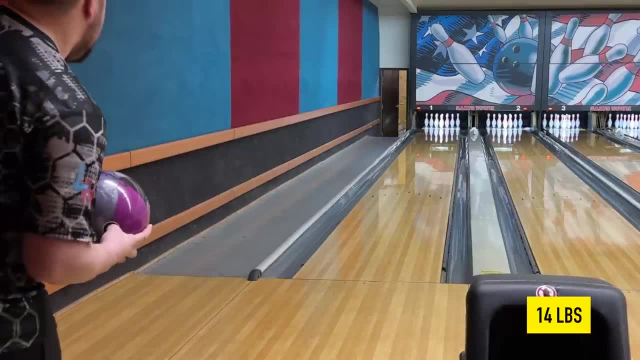 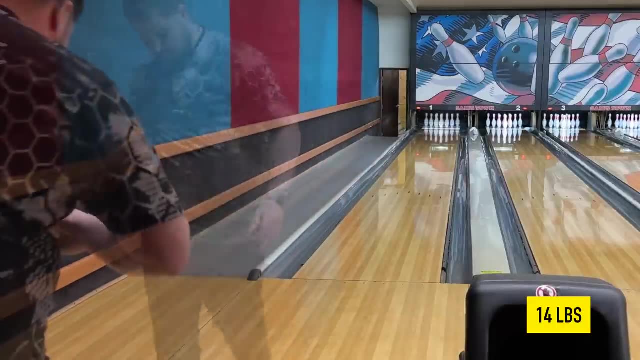 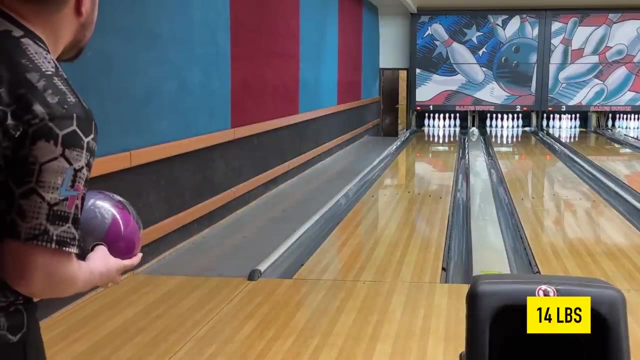 Oh, Oh, Let's make a better shot here. Good shot, All right. last shot of the video here. After here, I'm going to do some quick math, figure out some averages and we'll get to the desk. Oh. 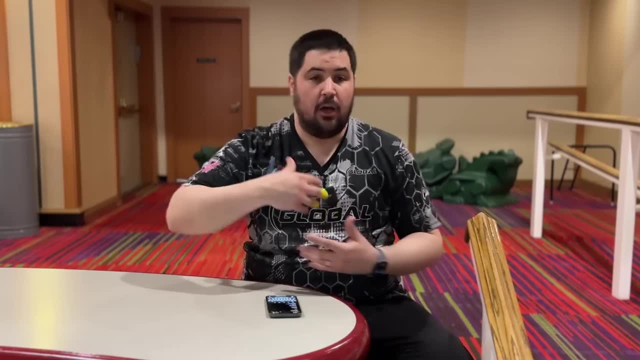 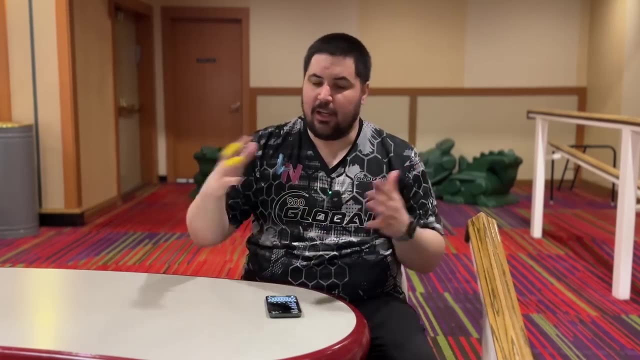 All right, so now we're all done done, kind of comparing the 14 pound versus 15 pound. is it going to be a higher rev rate, lower rev rate, higher speed, lower speed, carry percentage, all that stuff. so my testing is only today's only. 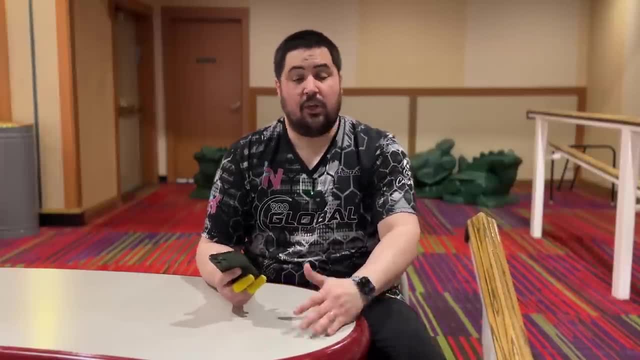 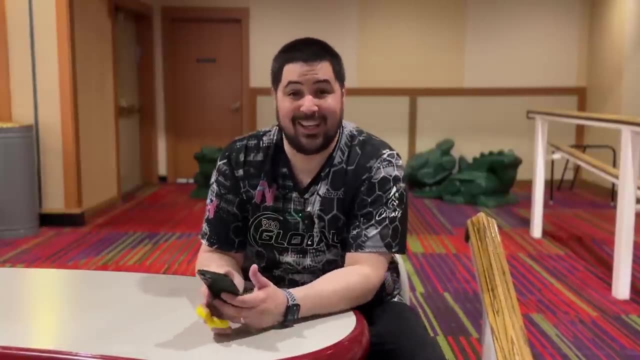 day one, i threw 18 shots with 14 pounds and i threw 18 shots with 15 pounds. nothing got cut. all the good shots, all the bad shots, because that's what bowling is, and i'm gonna tell you guys here. i got it on my my notes here. i'll screenshot it for you guys right now. put it on. 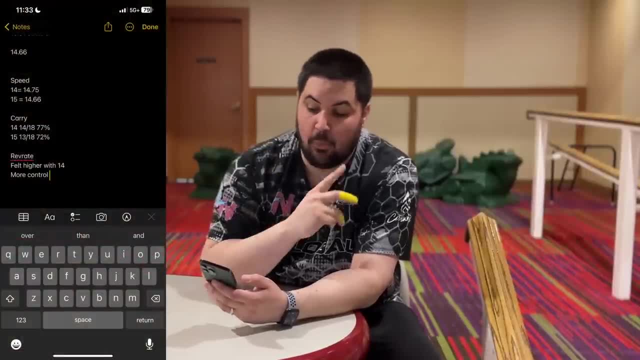 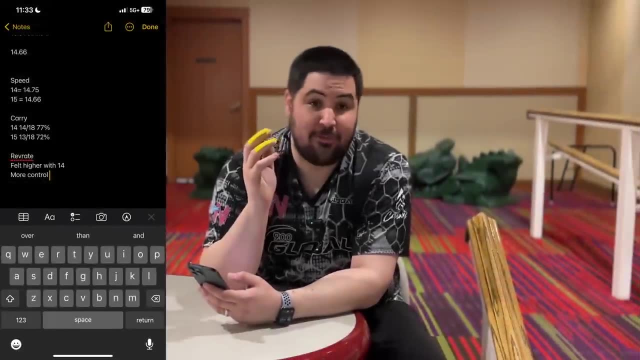 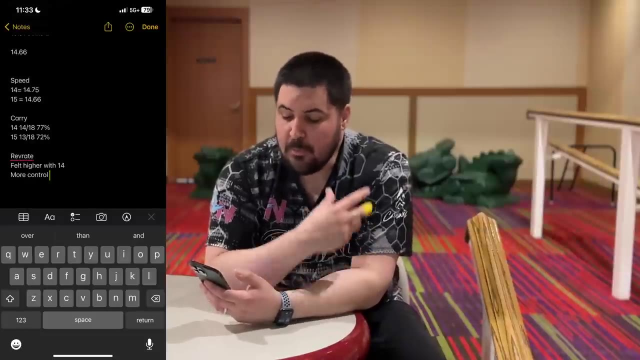 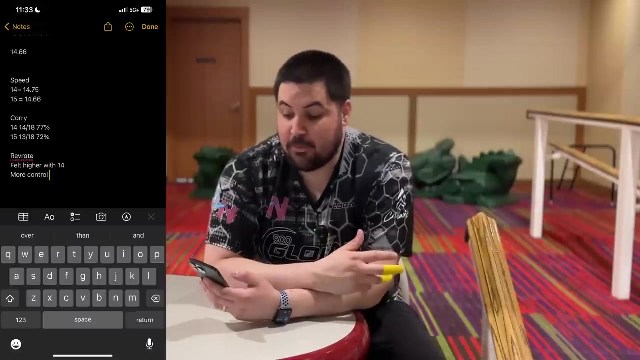 screen my speed. my average speed with 14 pounds was 14.75. okay, and the speed definitely dropped when i moved in and did my little slow hook. if not it would have been a little bit higher, closer to 15. but 14.75 was my average ball speed with 14. then when i went to 15, my average ball speed 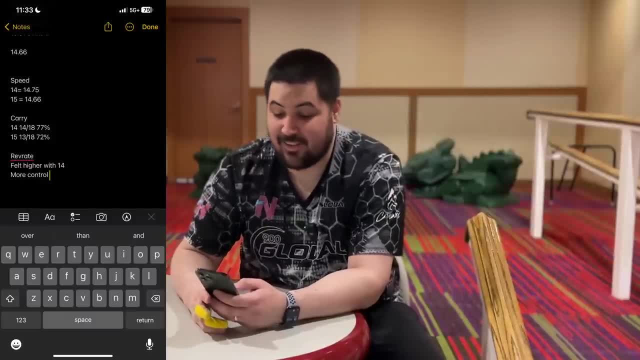 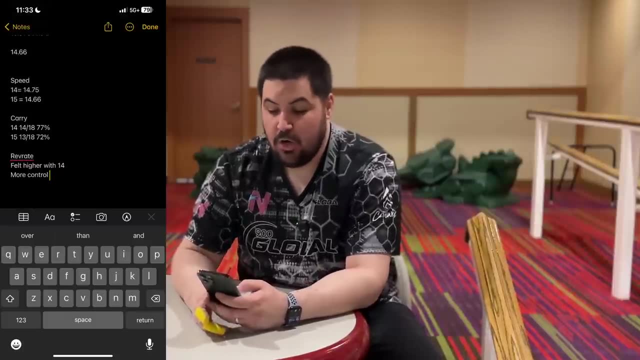 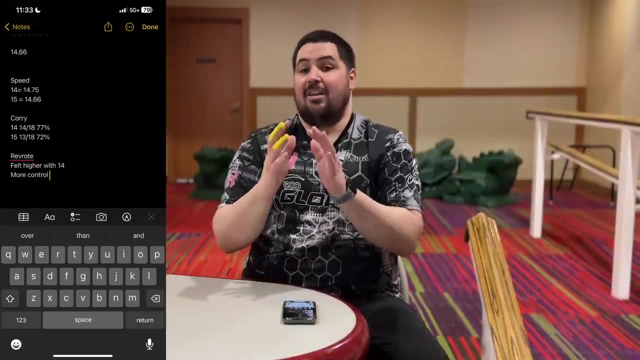 plummeted to 14.66. that's a difference of 0.09, so less than one-tenth of a mile per hour. so when we talk about ball speed, i was very surprised that that difference was only one-tenth of a mile per hour. and right from my first couple shots it did not feel like i was throwing the ball any slower or any faster. with the 14 pound ball it felt like that was just my normal speed and i was able to get into my swing and came down. and i feel like with the 15 pound ball it actually helped a little. 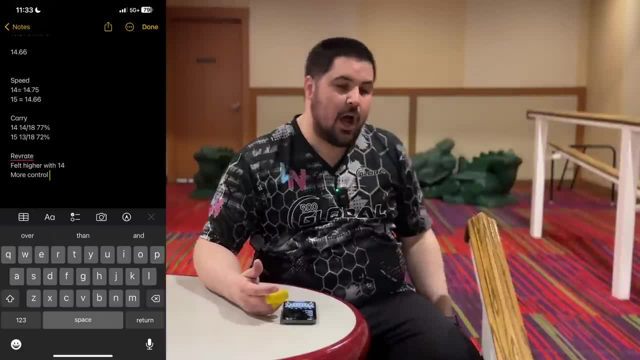 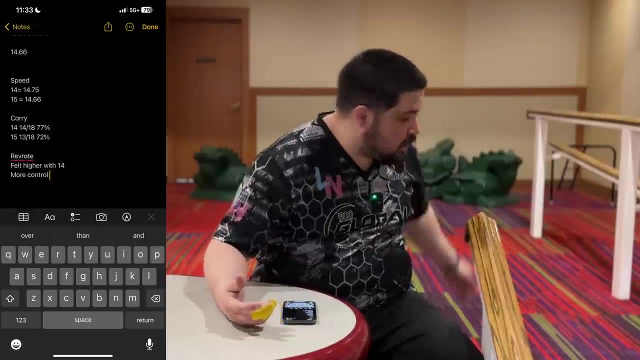 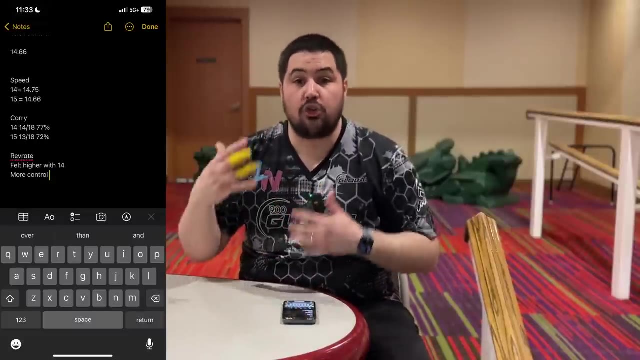 bit with ball speed because there's more weight coming down and that kind of tells me that my backswing is pretty free, because with the 14 pound ball it was less weight coming through. so i can see why the 14 went a little bit higher. i'm just very surprised that it wasn't a larger. difference. now, one thing that everyone always talks about is the carry percentage. everyone thinks that you want to carry more with 14 or with 15 versus 14 higher weight, yada, yada, yada, and i've always been on the camp that that's not true, because if higher weight yielded, higher carry. 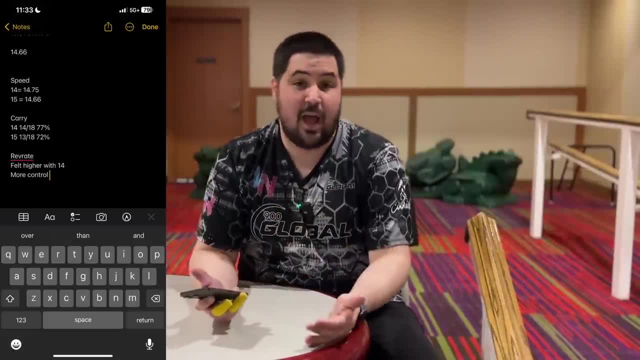 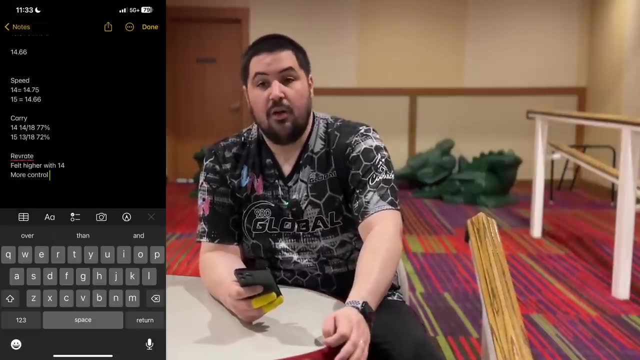 percentage. then all the pros would throw 16 and that's just not happening. so carry percentage: 14 pounds. i went. i struck 14 out of 18 for a 77 and i didn't flat 10 once. i, i, i 10 pinned once and it was a. 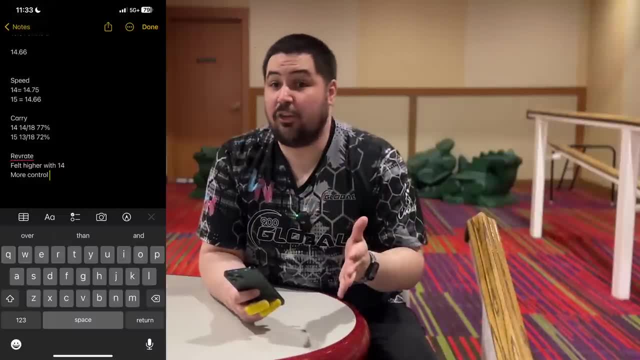 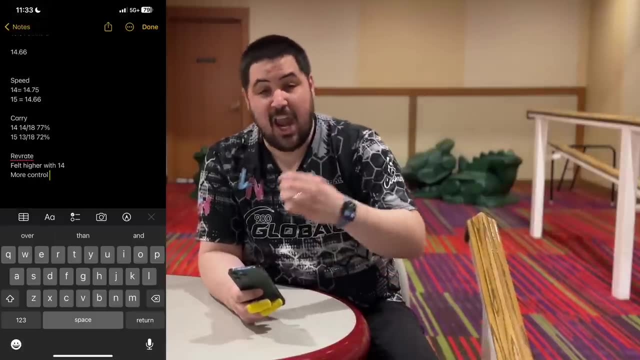 it wasn't a- well, i guess it was a shaker 10.. i seven pin twice, which could have very easily been strikes. then, when we turn it over to 15, i struck 13 out of 18 and i flat 10 twice. so if we're 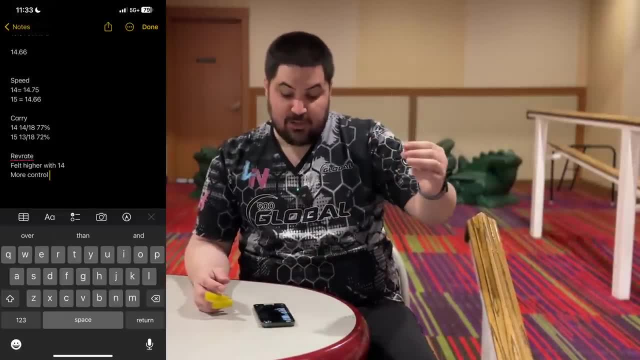 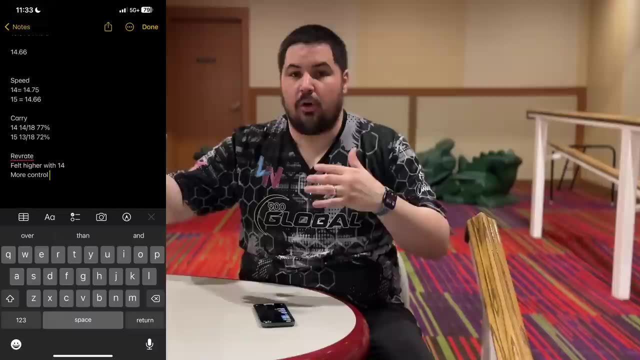 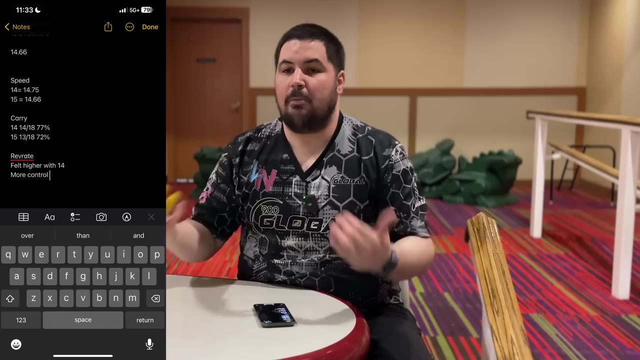 talking about a carry percentage difference. it went from 77 with 14 to 72 percent with 15, but i think it's the number is actually higher with 14 because i didn't flat 10 once and i think if you, that carry percentage number should be lower than if you blow a seven pin, if that makes any kind of 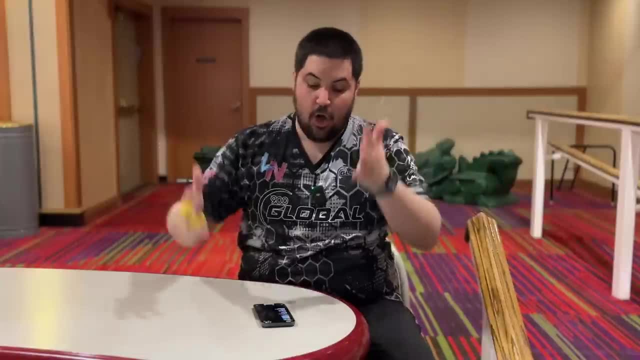 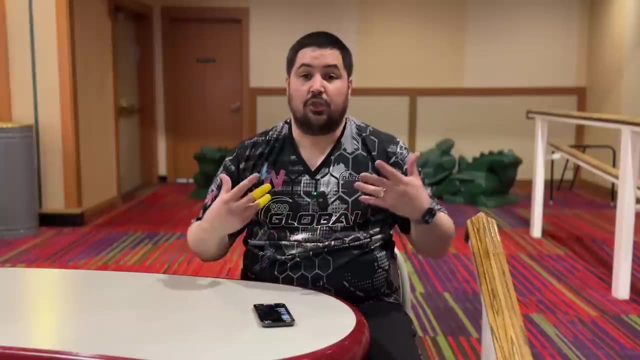 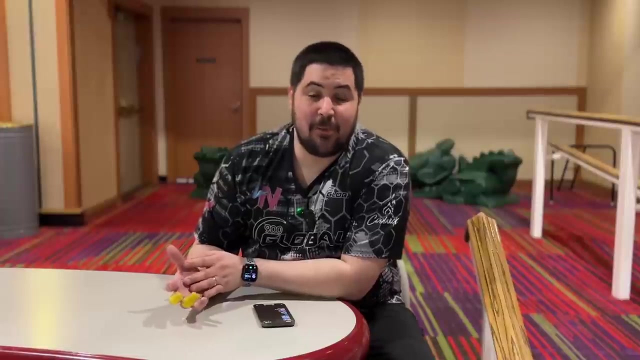 logical sense. in my brain it kind of makes logical sense and i hope you guys are seeing that rev rate. i don't have a way to gauge my rev right here, so you're just going to have to trust me on my feel, on my intuition. what i felt when i was bowling- and it did feel like my reverie was a little bit higher.